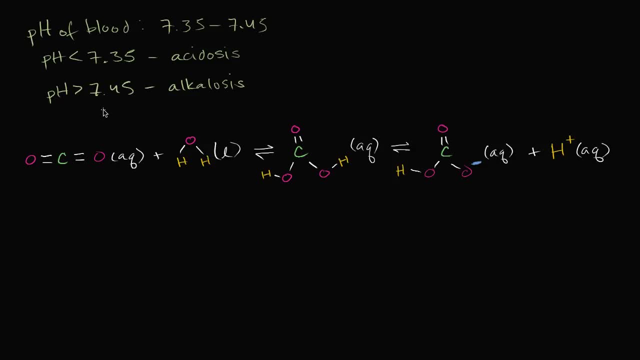 with acidic things, acidic molecules entering our blood or basic molecules entering our blood. How can it handle that without our pH being able, while keeping our pH in this range right over here? And the answer lies in something that's also useful for the transportation of carbon dioxide in our blood. 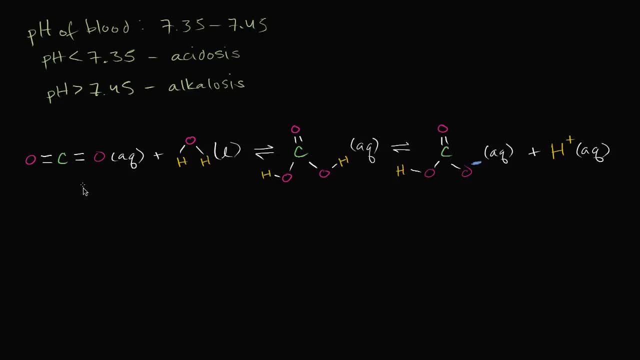 And this right over here, this, these equilibrium reactions. equilibrium reactions. we see that carbon dioxide, when you put it in the blood, which is primarily water, so carbon dioxide and aqueous solution- it will react and we have some enzymes. 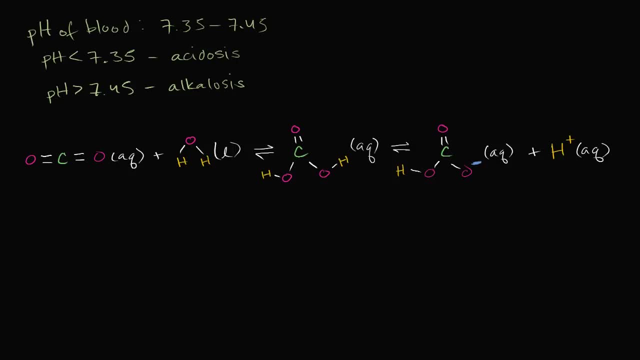 that help this, that help this along, but it will react to form carbonic acid. So let me write this down: It will react to form carbonic acid, which is a weak acid. This is carbonic acid And then that can dissociate to form bicarbonate. 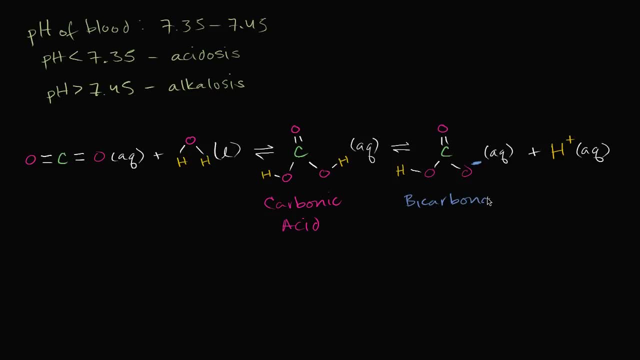 So let me write that over here: bicarbonate And a hydrogen ion, or when we know that that would just attach to a water molecule and become a hydronium ion. And so why is this useful? Well, I said, it's actually part of the carbon dioxide. 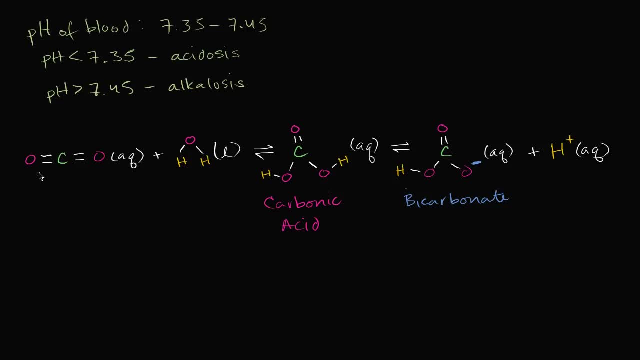 transportation in the blood, because, based on the sources I've looked at, about five to 10% of your carbon dioxide can just dissolve in the blood, and then also another roughly five or 10% can actually be bound to hemoglobin and be transported that way. 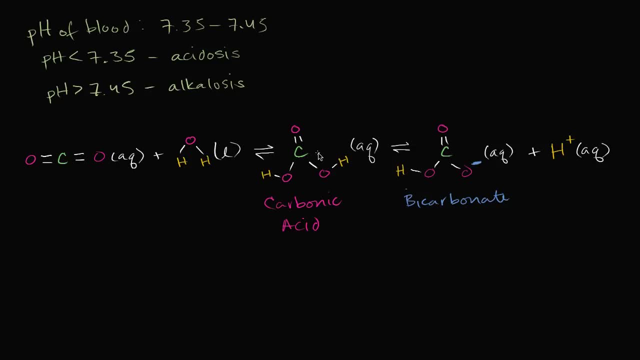 But the bulk of it actually needs to go through, needs to actually be transformed, needs to react to become carbonic acid and bicarbonate in order to be transported, In fact, in your blood. most of the carbon dioxide in your blood is actually in this form, right over here. 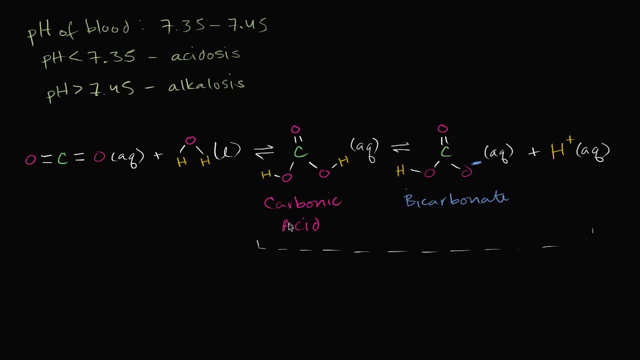 and, in particular, bicarbonate And the sources. I look at it, 80 to 90% of the carbon dioxide in your blood is being transported in these forms, and primarily as bicarbonate. So this isn't the topic of this video. What's a useful way to transport carbon dioxide? 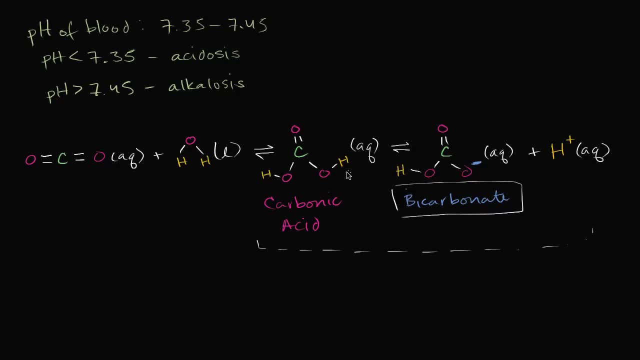 in your blood, but this is why this is how we do it. But the topic of this video is why this is also useful for maintaining our blood pH in this range, Because these equilibrium reactions between carbon dioxide, carbonic acid and bicarbonate- this is a buffer system. 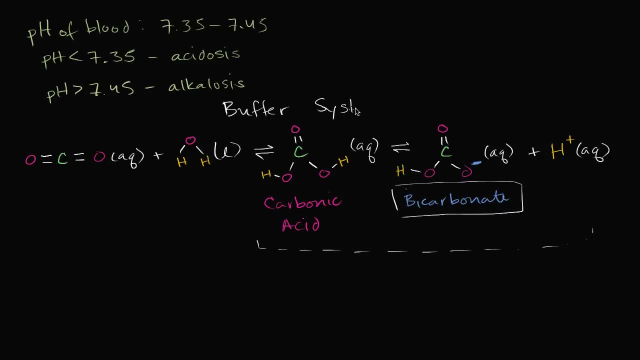 This is a buffer system And the word buffer- in our everyday language it refers to something that kind of smooths the impact of something or it reduces the shock of something, And that's exactly what's happening here. Let's think about, remember, these are all equilibrium. 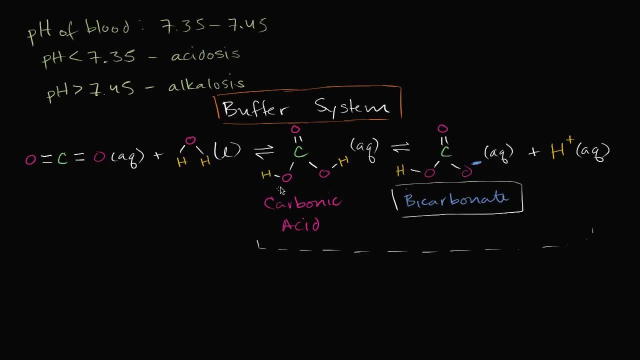 reactions. this is a weak acid and you can even look at the different constituents of these molecules and account for them. You have one carbon here, one carbon here, one carbon there. You have one, two, three oxygens there. You have one, two, three oxygens there. 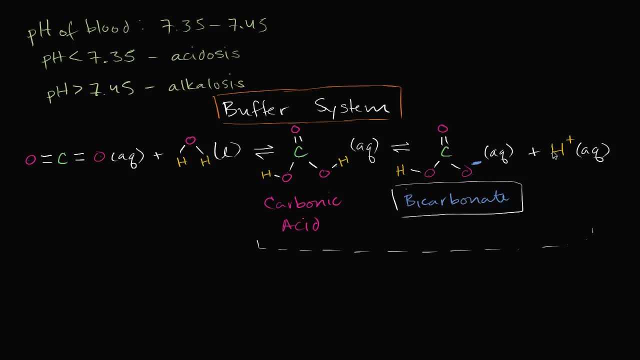 One, two, three oxygens. there You have two hydrogens, two hydrogens, two hydrogens. But let's just think about what if you had a carbon dioxide system? What if you started dumping hydrogen ions in the blood? So what if you were to dump hydrogen ions? 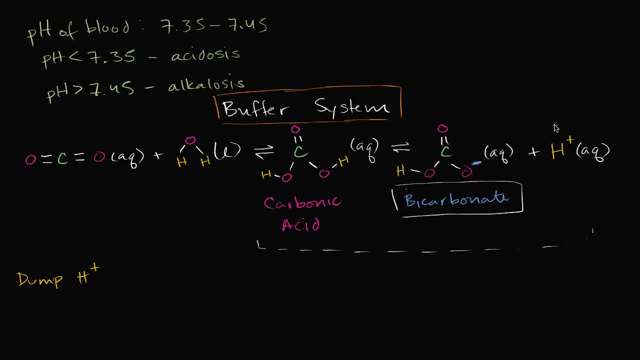 What's going to happen? Well, if you dump more hydrogen ions, if this right over here increases. well, actually, let me put it this way: If you were to just dump hydrogen ions and if you didn't have this buffer system, then your pH would decrease. 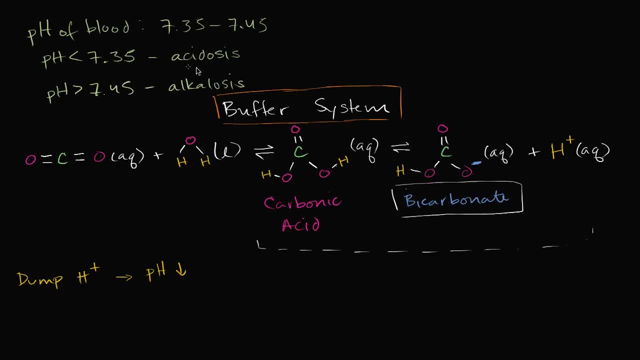 Your pH would go down and if you do it, enough your pH, you would end up with acidosis. Lucky for us, we have this buffer system, And so if you increase your hydrogen ion concentrations, Le Chatelier's principle tells us: hey, these equilibrium. 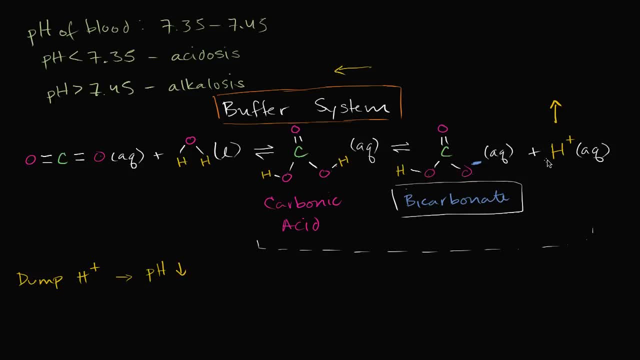 reactions are going to move to the left. So the more hydrogen ions you have sitting in the blood, the more likely they're going to bump into the bicarbonate in just the right way to form carbonic acid. And the more carbonic acid that you have in the blood well, 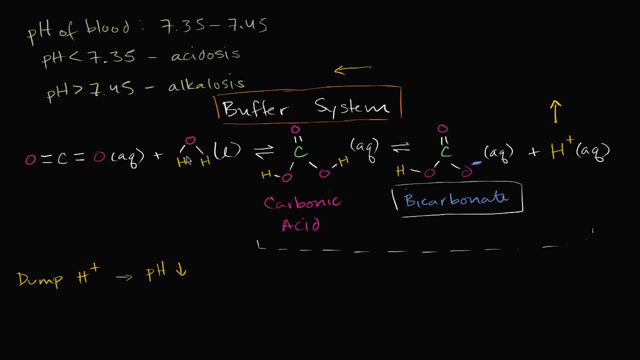 it's the less likely that you're going to have the carbon dioxide reacting with the water to form more carbonic acid. So as you add more hydrogen ions, they're just going to be sopped up by the bicarbonate. So this set of equilibrium reactions is going to move to. 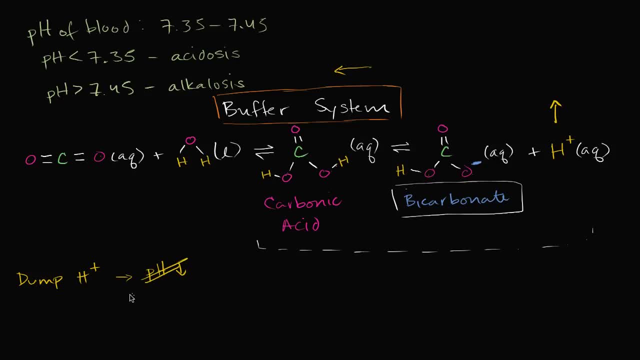 the left, so you're not going to have as big effect on pH. And similarly, if you dumped some base- let's say you dumped some base in your blood right over here- well, instead of just making your pH go up and possibly give you alkalosis-